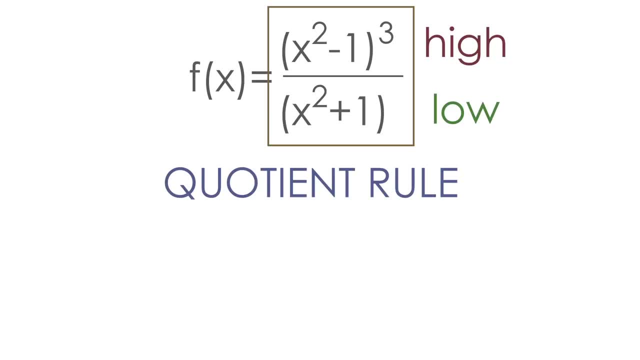 the x squared plus one the low, And now we can use the quotient rule formula to take the derivative And the formula is: low d high minus high d low, all over the square of what's below, And what this means is the low multiplied by the derivative of the high minus the high times, the derivative of 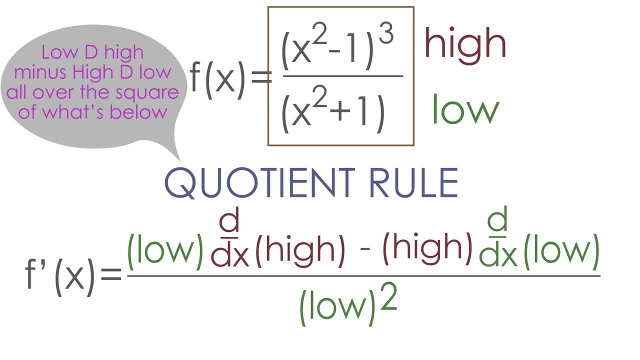 the low All divided by the low squared. All right, So now, at this point, the only thing we have to do is plug everything into our formula. So I'm going to plug in x squared minus one- cubed into everywhere we see the word high- And I'm going to plug in x squared plus one. 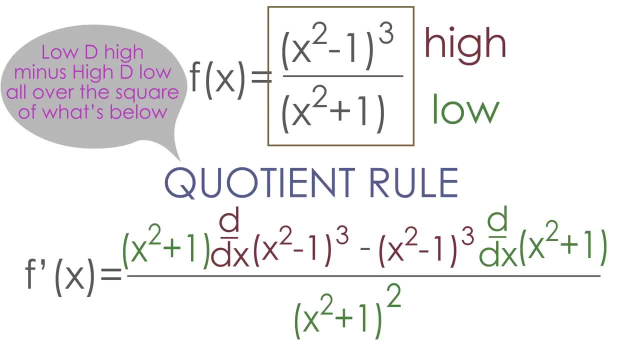 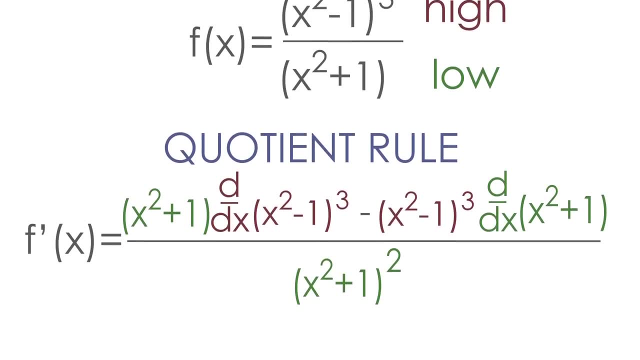 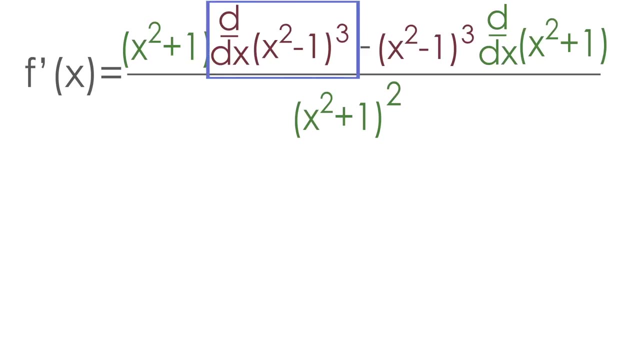 into. everywhere we see the word low, And at this point the only thing we have to do is simplify this derivative as much as possible. So, to start off, let's take the derivative of x squared minus one cubed. Now notice how we're. 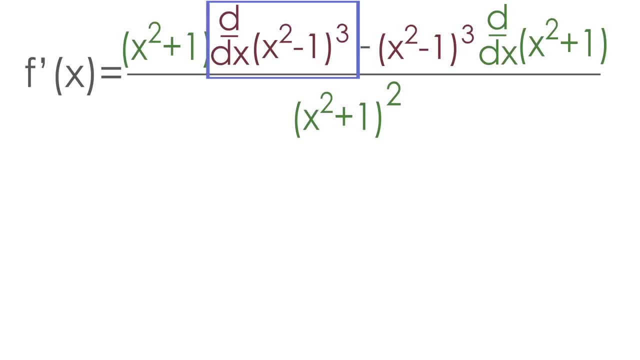 taking the derivative of a parentheses followed by an exponent of three. Parentheses followed by exponent means that we have to use the chain rule to take the derivative. So let's do this. Let's use the chain rule. The first thing we'll do is take our exponent of three and bring it to. 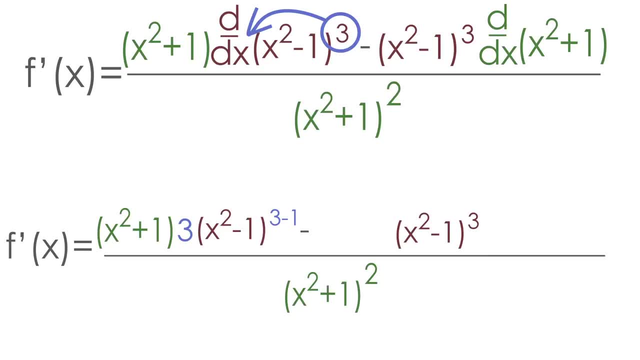 the front and multiply it in front of the parentheses, And our new exponent is going to be subtracted by one. So three minus one is equal to two. And now we need to use the chain rule, which means we have to multiply everything by the derivative of the inside of the parentheses. So the derivative 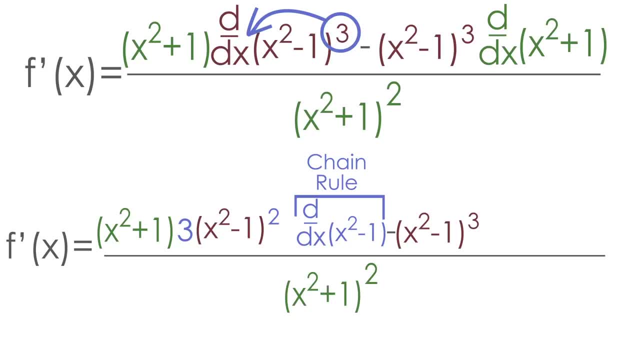 of x squared minus one, and the derivative of x squared is just two x. derivative of negative one is equal to zero. So this is just going to be equal to two x. All right, And so now let's move over to the right side of our equation And let's take 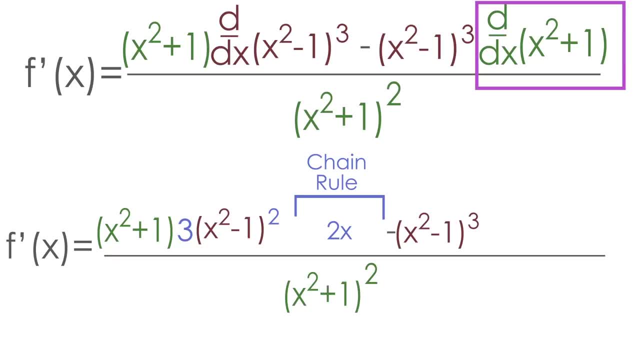 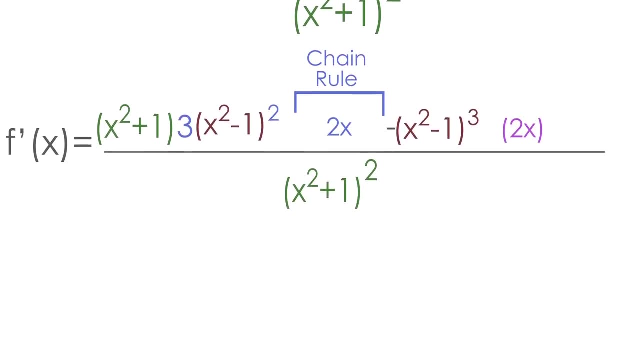 the derivative of x squared plus one. Now the derivative of x squared is just two x. The derivative of one is zero, So this is just equal to two x. All right, So now we have some algebra to simplify this derivative even further. The first thing we can do is multiply the two x. 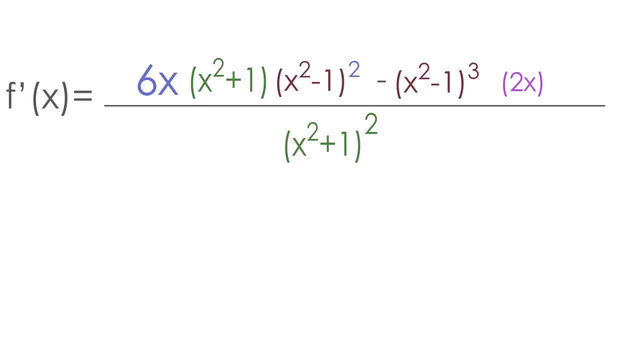 into three. Two x times three is equal to six x, And I will put this in the front. All right, So now, at this point, we can factor And notice how in the front term we have a six x And in the back term, 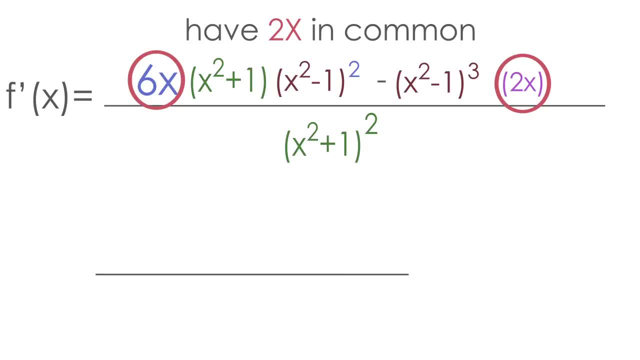 we have a two x, So they have a two x in common. that we can factor out. And also notice how the front term has two x squared minus ones And the back term has three x squared minus ones. So they have at least two x squared minus ones in common. So we can factor out. 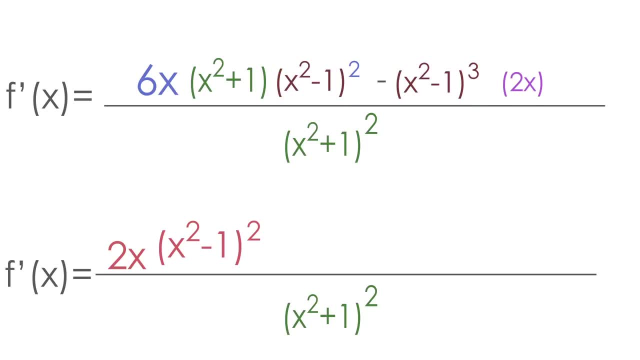 x squared minus one squared. All right, So now that we've factored, what do we have left? All right, So what we did was we ran out of numbers for both expressions And we just take the two x squares and the little tick together and we just cut them inside out. 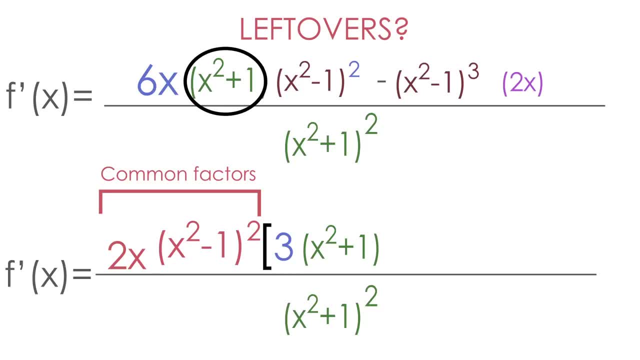 Finally, we take the two plus three plus x squares and we, Mother's Day, raise them up for the first person that's left over in each of our terms. In our first term we started with a six x, But we factored out a two x, So we have a three leftover, The. 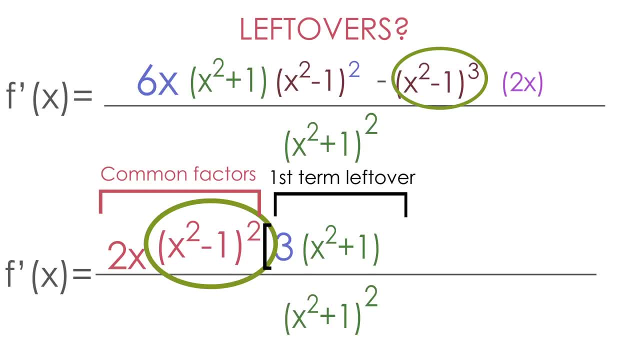 x squared plus one stays the same, since we did not factor out an x squared plus one. So we have 1 left over, but you never put a 1 exponent, so this just becomes x squared minus 1.. And the 2x will go away because we factored out a 2x already. 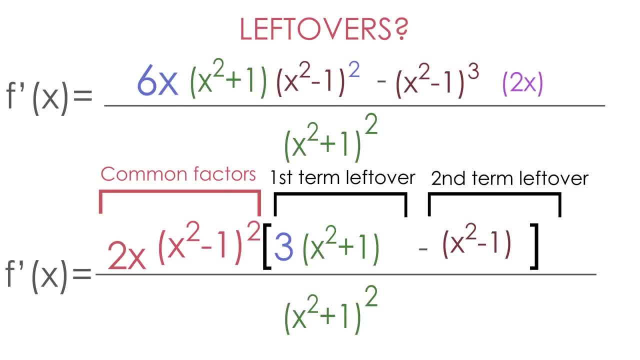 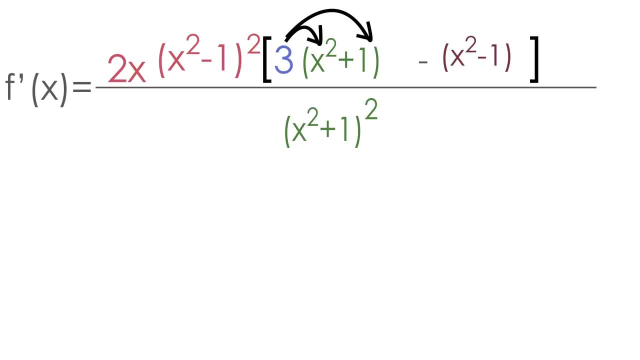 So we're just left with x squared minus 1 for our second term. All right, so now what I'm going to do is multiply the 3 with the x squared plus 1.. So 3 times x squared is equal to 3x squared. 3 times positive 1 is equal to positive 3.. 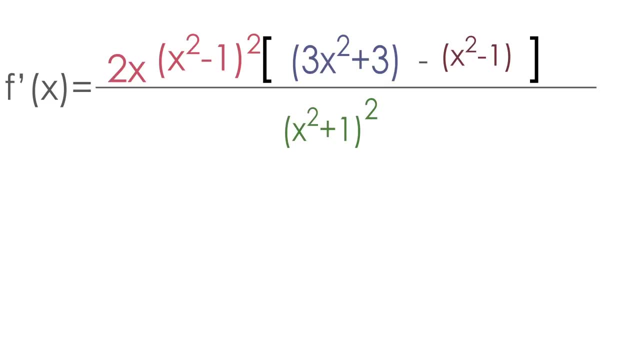 And at this point we can get rid of the parentheses of the 3x squared plus 3, because there's no negative sign in front of that parentheses. so this just stays the same: 3x squared plus 3.. And the next parentheses of x squared minus 1 does have a negative sign in front of it. 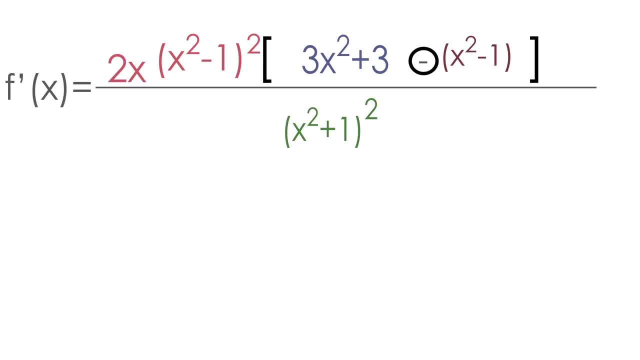 So this means all of the signs will switch, So the positive x squared becomes a negative x squared And the negative 1 becomes a positive 1.. All right, now that we got rid of our parentheses, now we can combine our like terms.